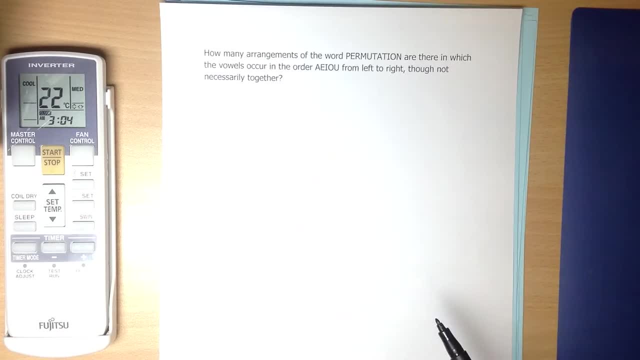 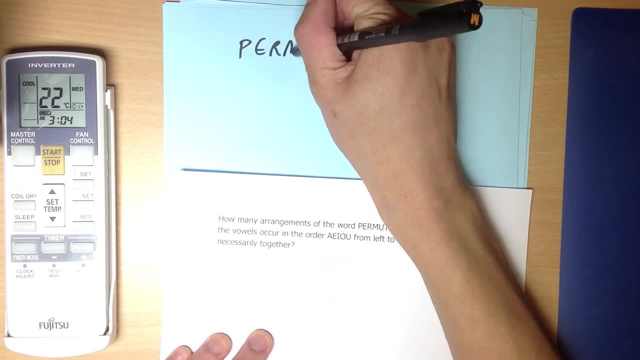 And not just can you, you know, pluck out random numbers, which will get you the right answer at the end. So here we go. The word permutation. let's just think about that for a second Before you think about the vowels. okay, 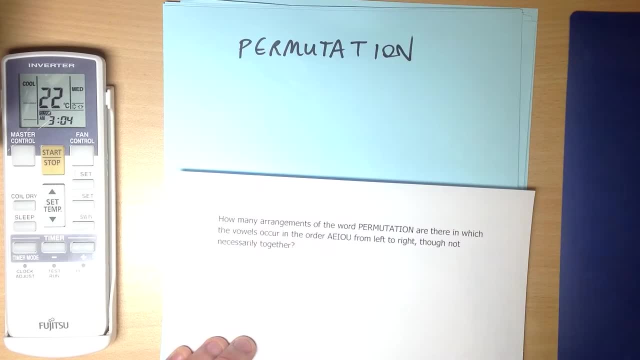 The word permutation has 1,, 2,, 3,, 4,, 5,, 6,, 7,, 8.. 9, 10, 11 letters- okay, 11 letters, right. So the first thing I would set out is that, forgetting about what the letters are, right. 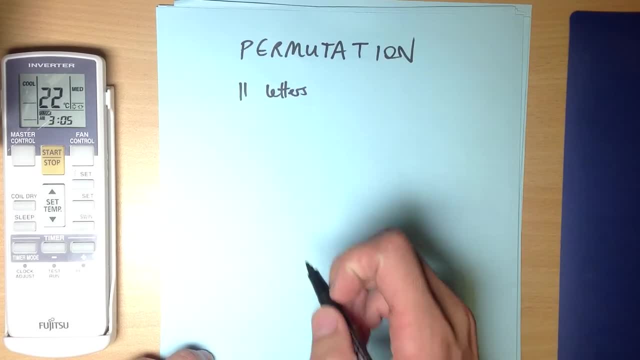 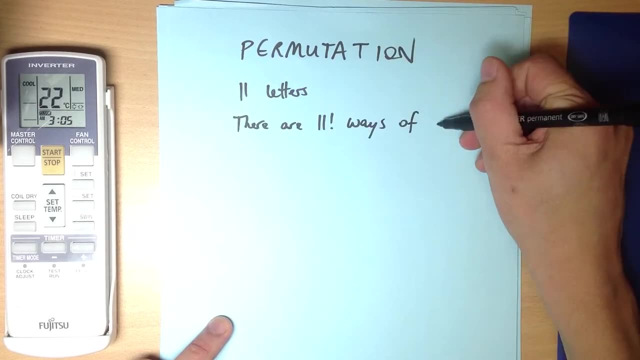 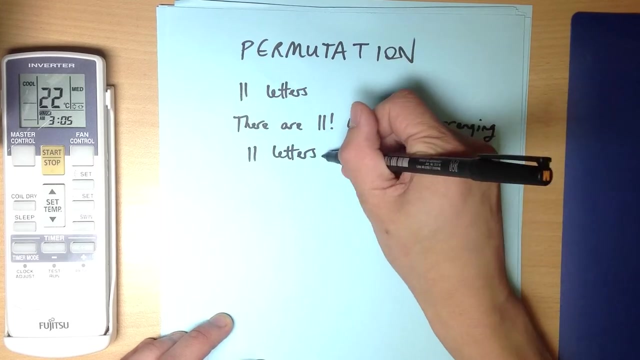 And any kinds of conditions on them. I'm going to add conditions as I go. I'm going to say there are 11 factorial ways of arranging 11 letters. So that's pretty sort of standard arrangements, before you even get to permutations and combinations. 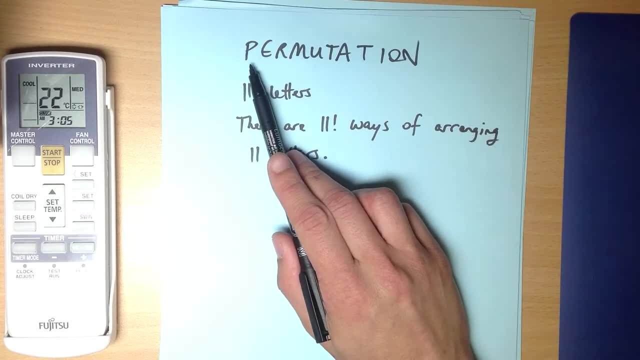 As a topic. you've got, you know, 11 slots, and how many letters can you? how many choices do you have for the first slot? You've got 11, because you've got 11 that haven't been picked. 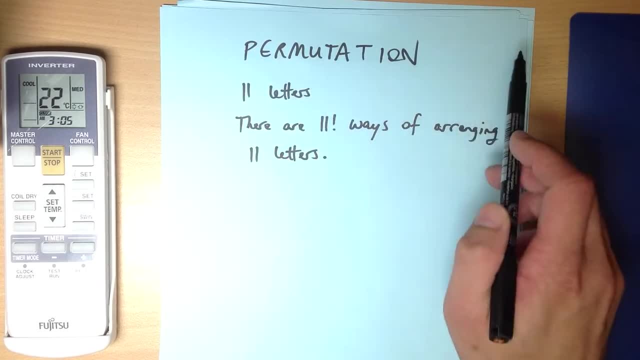 Then how about the next one? Well, you've got 10 left and then 9, and so on. So when you multiply them all together, you get 11 factorial okay, Right, so this is kind of our baseline, right. 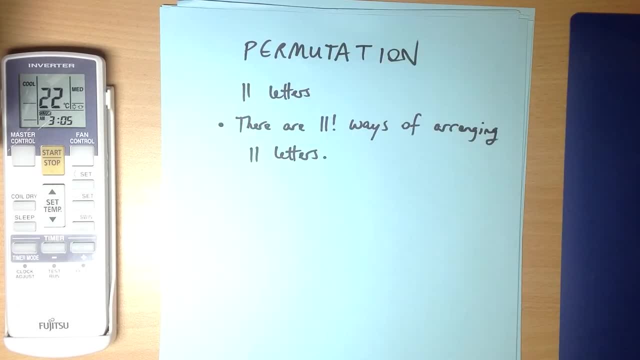 This is my first thing which I'm going to say, And I'm now going to try and drill down and become more specific and add conditions on okay. So let's think about the next thing Now, when you have a think about all of the arrangements that you're going to get, these 11 factorial arrangements, massive number, okay. 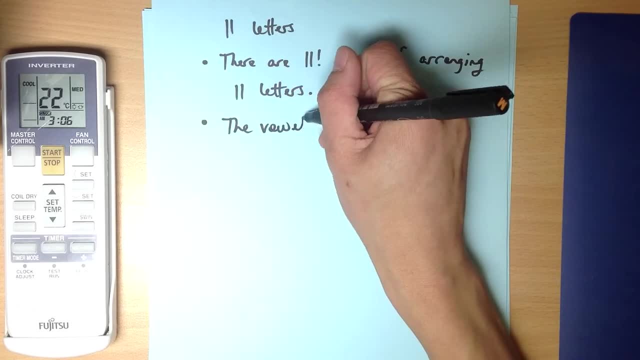 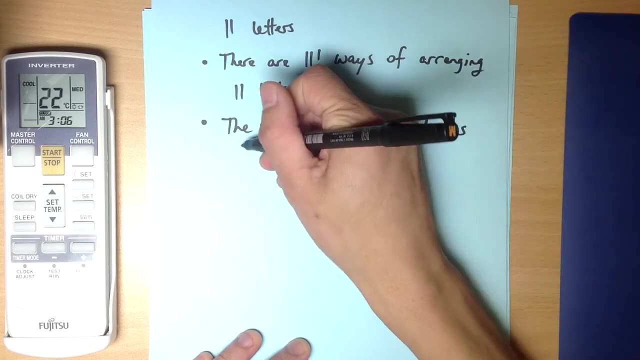 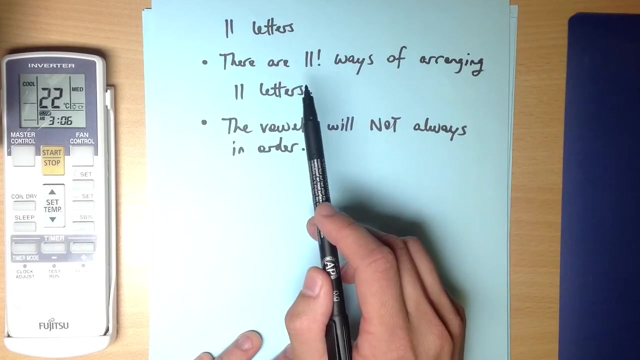 In these arrangements, the vowels will not always be in order. So that's a bad thing for us, right? Because we only want the ones where the vowels are in order, okay, So how many of these 11 factorial arrangements ways? how many of them have the vowels in order? 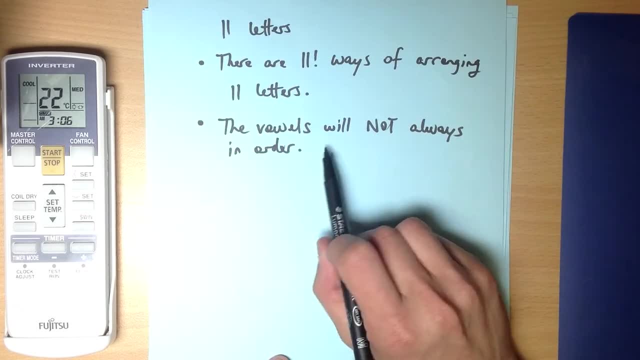 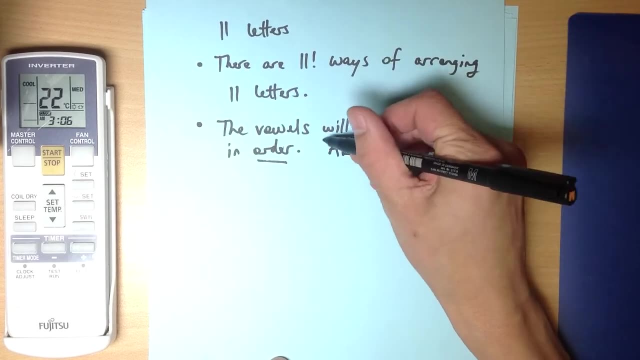 Well, to answer. To answer that, I want to think about how many different ways are there to get the vowels right, How many different ways are there to order the vowels? And the answer is because there are 5 vowels: A, E, I, O, U, right. 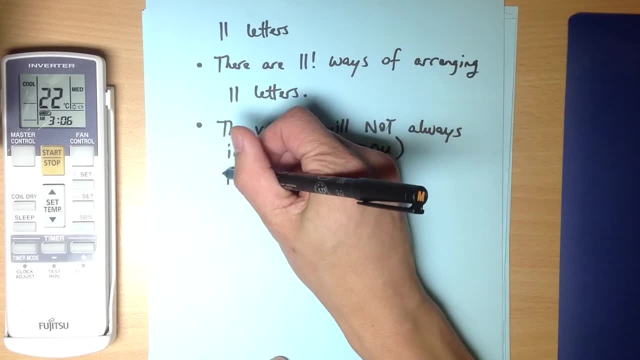 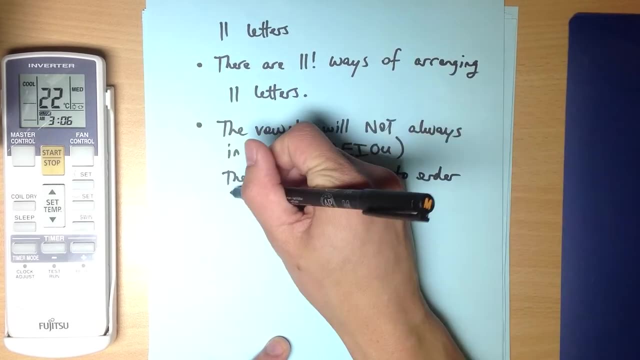 How many ways are there to reorder them? Well, the answer is there are 5 factorial ways to order the vowels right Now. here's the thing: Out of those 5 factorial, What's that? I think it's 120 off the top of my head. 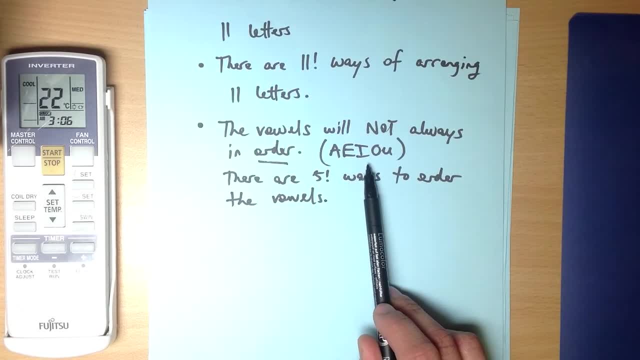 Out of those 5 factorial. Out of those 5 factorial. Out of those 5 factorial ways, how many of those ways am I interested in? And the answer is: I'm only interested in one way: the specific way where all of the vowels are in this order, and this order only okay. 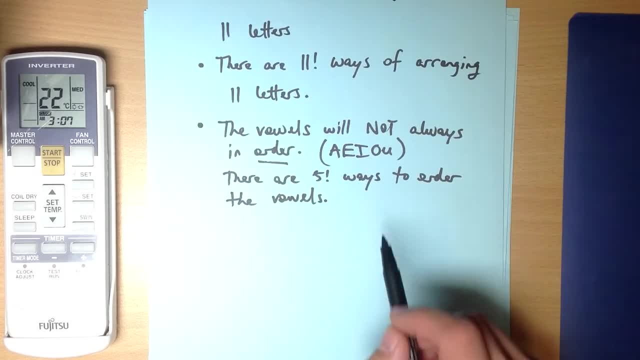 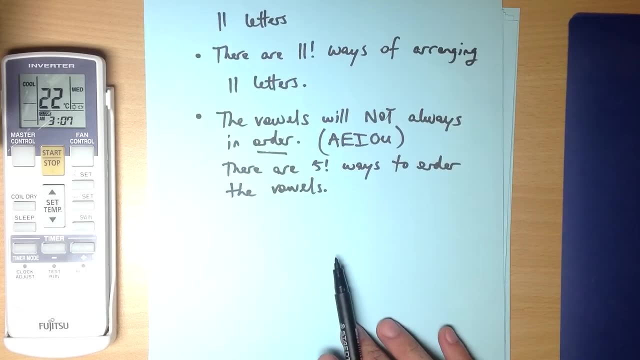 So since there are 5 factorial, 120 different ways and I'm only interested in one of them, right, That means I've over-counted by a factor of 5 factorial or a factor of 11 factorial, sorry, 120, right. 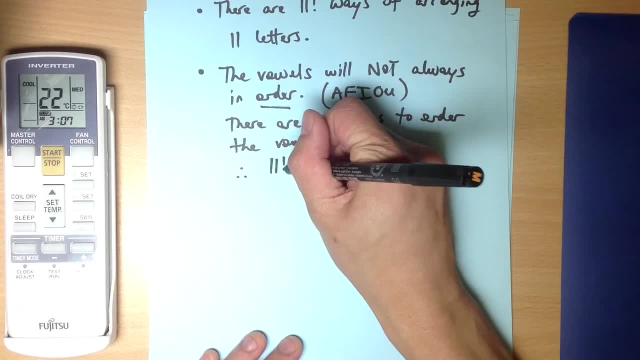 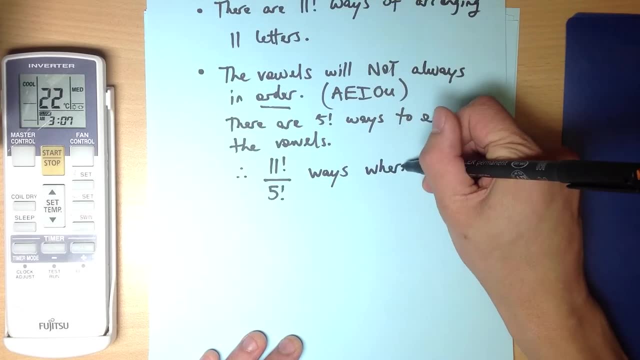 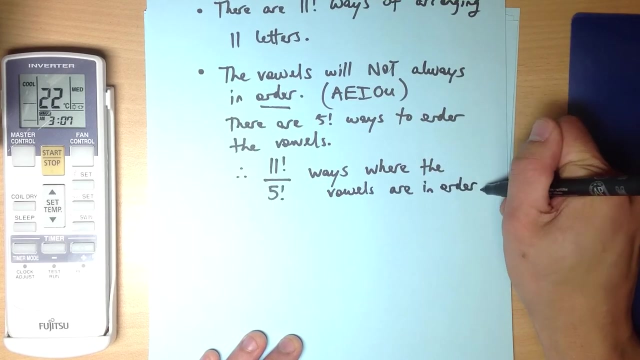 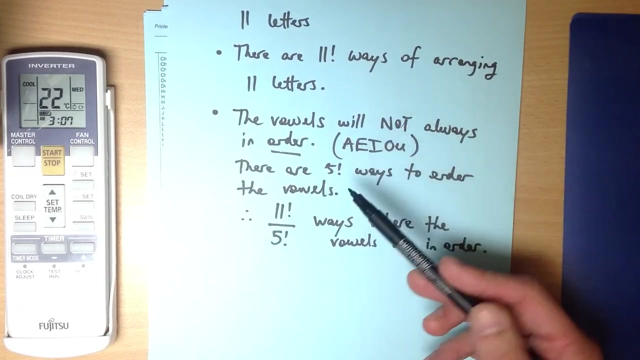 So therefore there are 11 factorial divided. So therefore there are 11 factorial divided by 5 factorial ways, where I've got 11 letters and the vowels are in order. okay. So can you see how- because I've over-counted in my original calculation to compensate, I divide right. 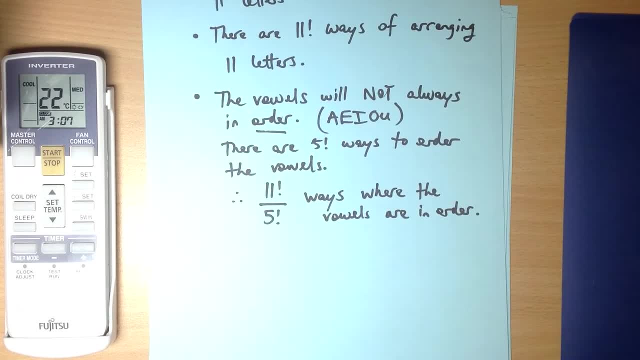 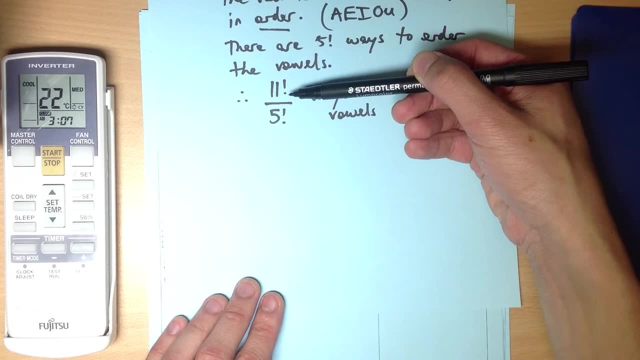 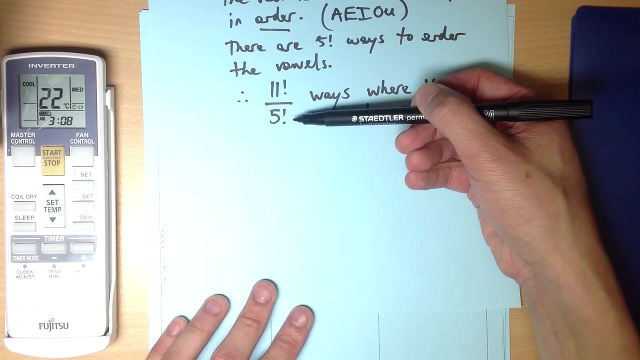 That'll divide me down and get 5 factorial less as a factor ways of arrangements, okay. So now I've got so far this is an 11-letter word right with 11 letters to choose from. Now I've narrowed down that I only want the ones where the A, E, I, O and U are in order, okay. 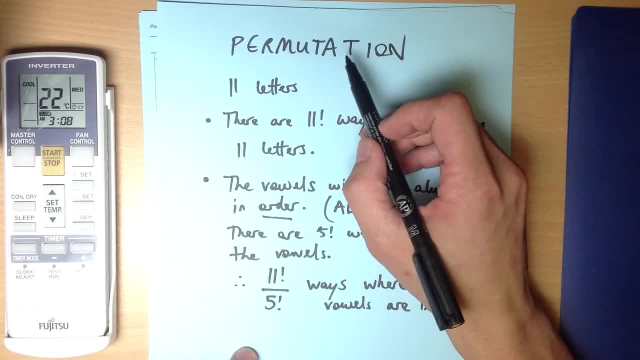 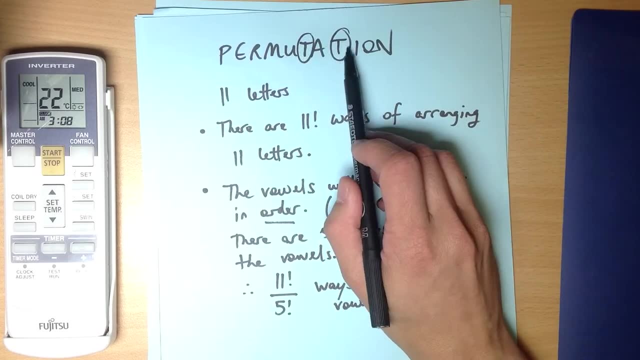 Now I have to think about: are there any other limitations? And the answer is yes, because in my word two of the letters are identical. okay, the two Ts. Now that means that I can arrange those two Ts in two factorial ways. 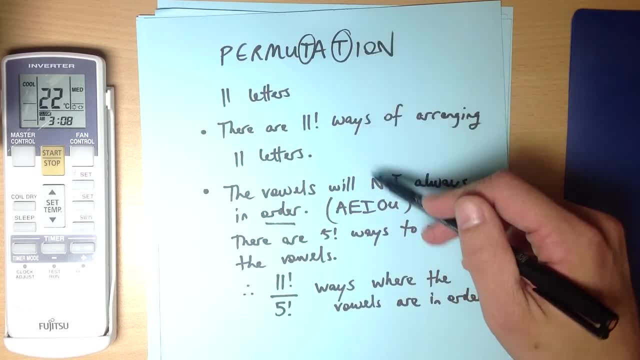 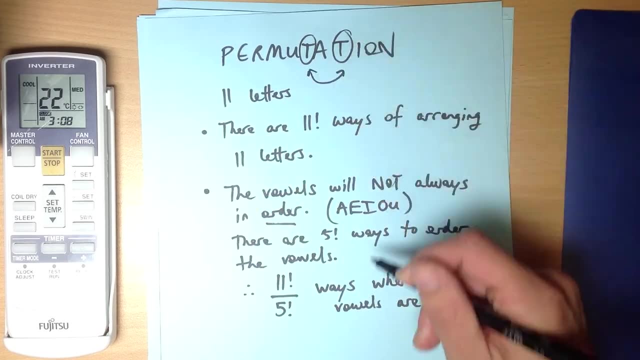 If I had three Ts, it'd be three factorial more. So again, I've over-counted, because this permutation, this way of spelling it, if I swap these two Ts around would look exactly the same, But this way of counting would double them up right. 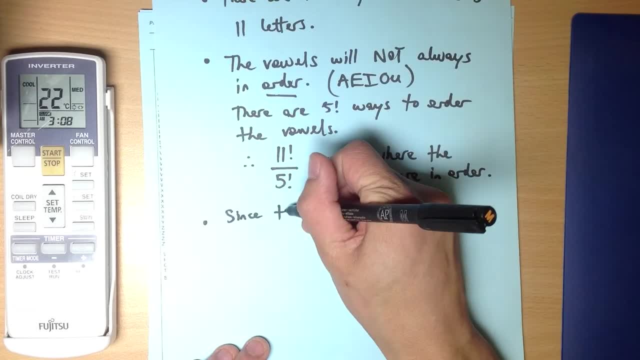 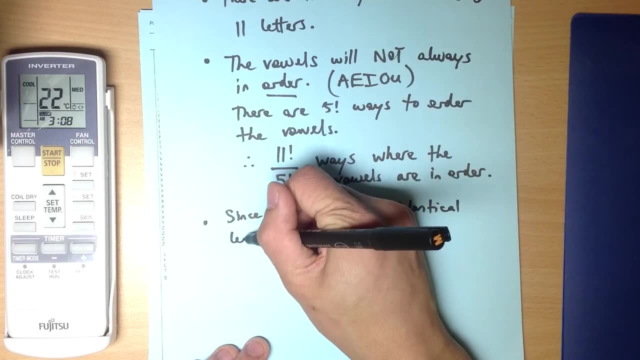 So, therefore, since there are two identical letters, right and again, like I said, I'm actually going to write this down as part of my answer, Because it demonstrates that I know where the numbers that I'm writing are coming from, right. 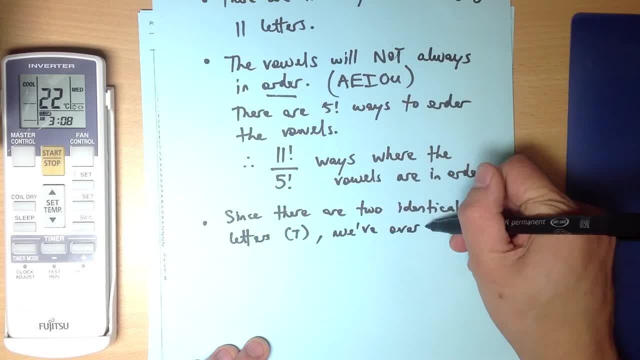 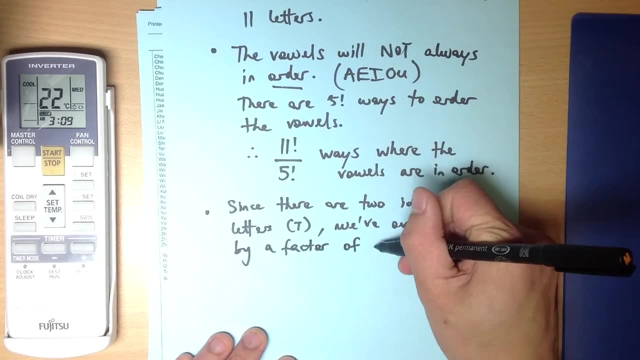 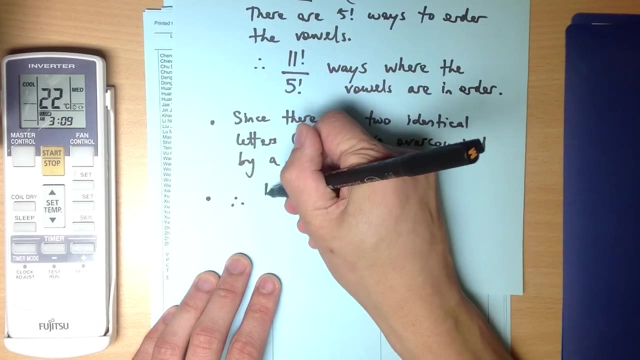 We've over-counted by a factor of two factorial. okay. So just like with the five factorial before, I have to divide through by that right, And this is all the conditions, right? So therefore there are 11 factorial on five factorial, two factorial ways.